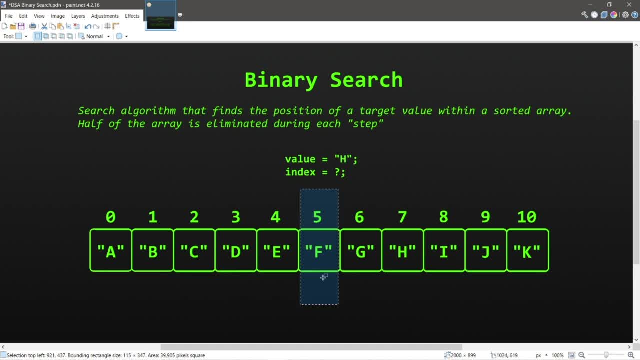 We first check to see if our target value is equal to this middle value. If these are equal, then we can return this index. But odds are they're probably not going to be equal on the very first turn, the very first step. So these are not equal. Then we will check to see if our target value is. 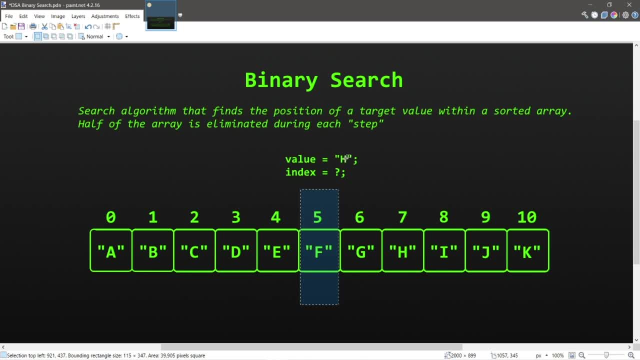 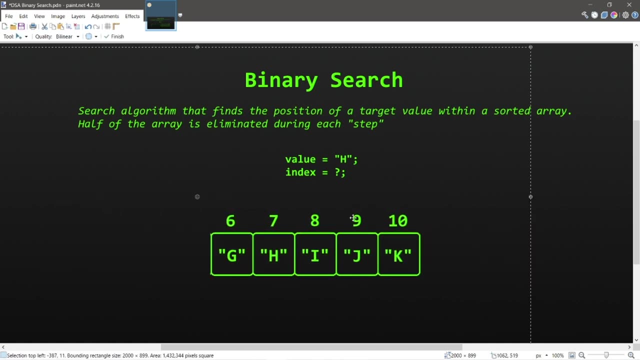 greater than or less than this middle value. Since H is greater than F, we can disregard this entire first half of our array because, since this is sorted, our target value could not possibly be within this first portion. And then we begin step two, or phase two. It's the same process as before. 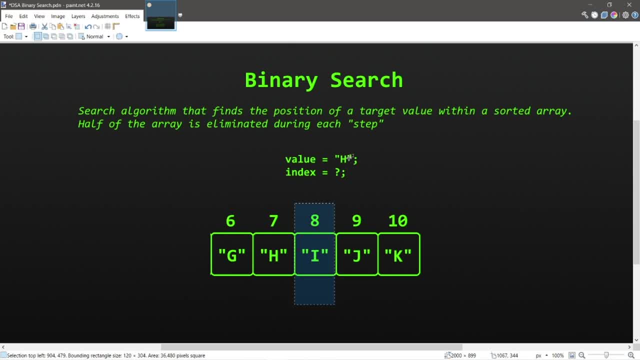 So again, we begin in the middle. check to see if our target value is equal to the middle value. They're not Check to see if our target value is greater than or less than the middle value. This time H is less than I. We would delete the second half of this portion. 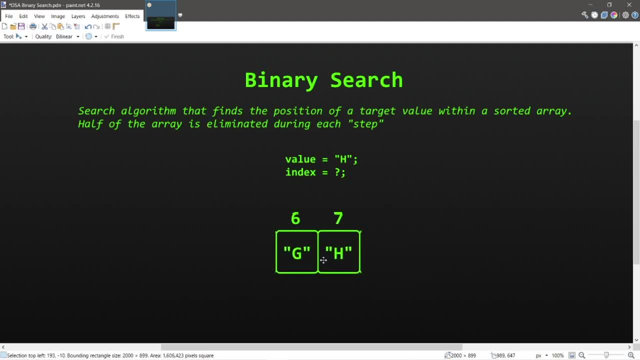 We're not actually deleting these values, We're disregarding them. And then we can move on to step three. We're repeating the same process as before, and this time these elements divide evenly. So we would just round down and begin and say that this is the middle. 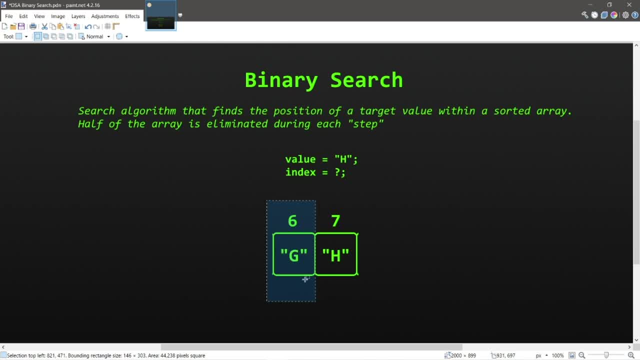 So h is greater than g. we would disregard this element and we only have h remaining. so we would return this index because these values are equal, and that's a binary search. Now, a binary search isn't too efficient when working with small datasets. however, if you're. 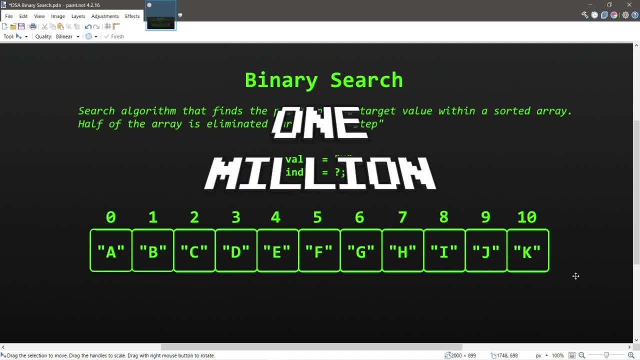 working with a large dataset like 1 million elements. well then, a binary search is actually fantastic, because we're eliminating half of the elements we are searching through during each phase or turn. So if we had a million elements after the first phase, we can already disregard. 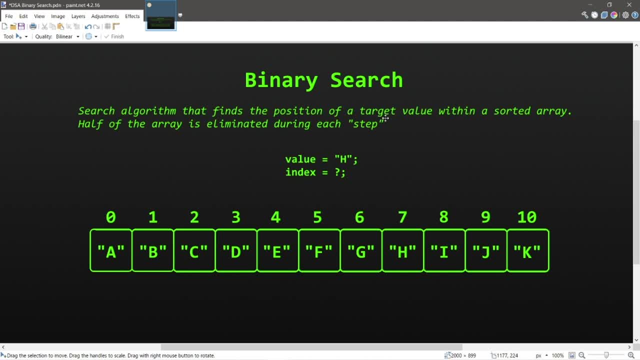 like half a million elements and then we just repeat the process until there's only one left. So if this was an iterative approach, we would need to search through these linearly, beginning with index 0 and going all the way to a million. So a binary search is fantastic with large 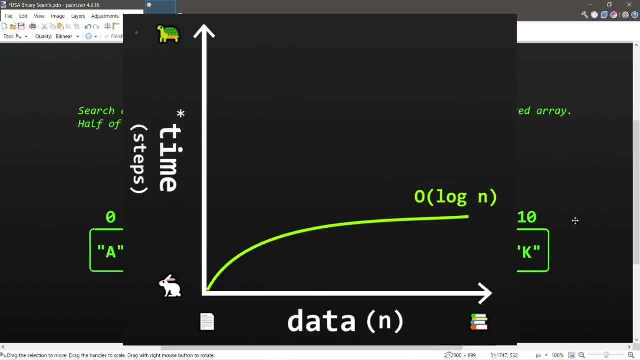 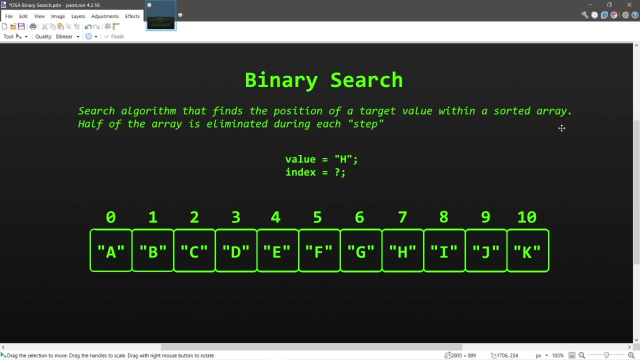 datasets. The runtime complexity of a binary search is O of log n. The larger the dataset, a binary search becomes a binary search. It becomes more and more efficient compared to other search algorithms. All right, let's perform a binary search in real life. now We'll use the built-in binary search. 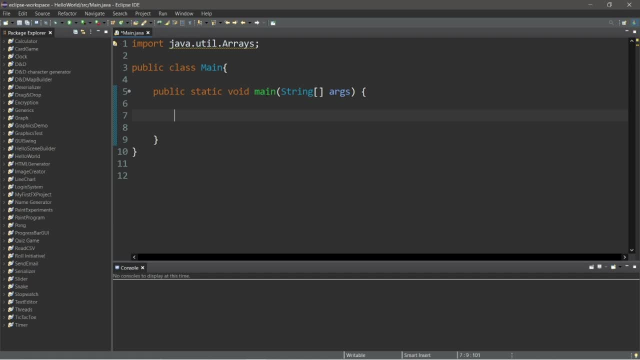 method of arrays to begin with, and then later on we'll build our own binary search function. So we'll need an array to work with. Let's say we have an array of integers named array, Int array, and the size of this array will be 100.. We'll increase the size later for demonstration. 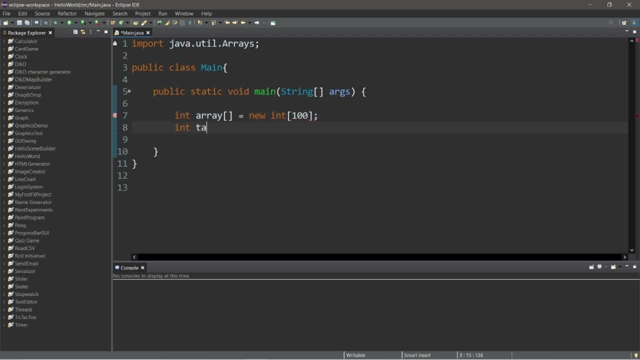 purposes, and we'll need a target value that we're searching for. I'll just name this target: Int. target Equals. what about 42?? We'll search for the number 42, and we'll need to populate our array So we can do so using a for loop. Int i equals 0.. We will continue this for loop as long as i is. 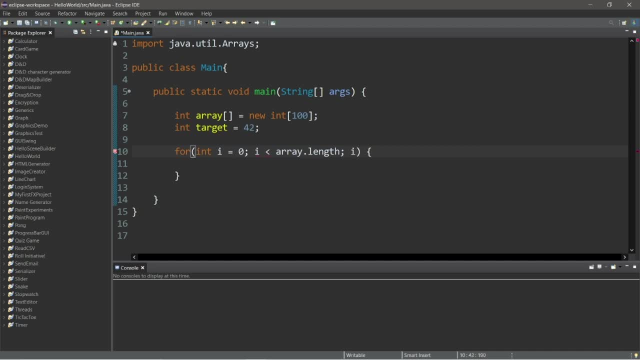 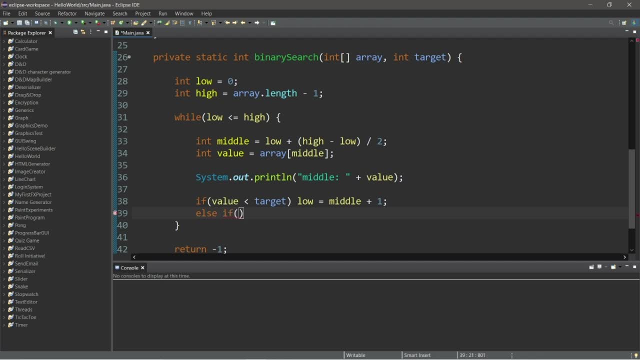 Okay, so the cheap way of using a binary search is to use a binary search. Okay, so the cheap way of using a binary search is to use a binary search. Else, if value is greater than target, we will set our high index. 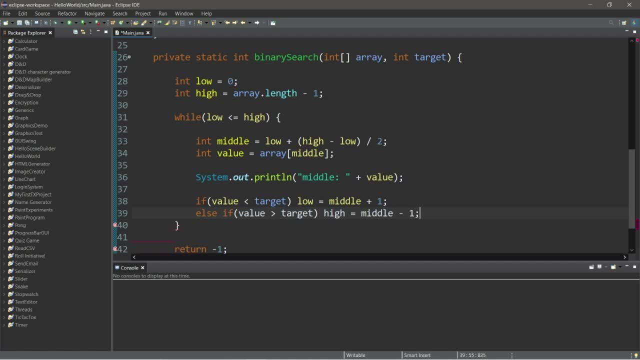 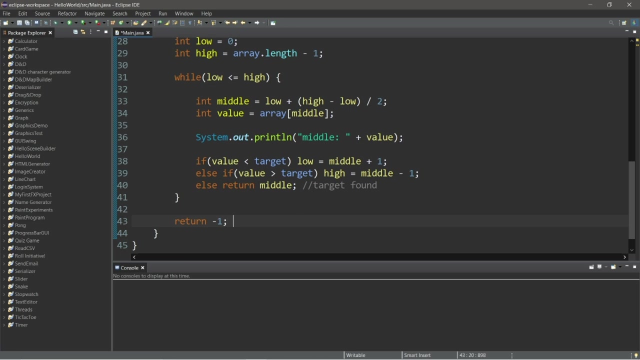 High equals middle minus 1.. Else, that means we have found our target. Else return middle, So this means that target is found. And by returning negative 1, that means target not found. And that is our binary search function. Let's try it. 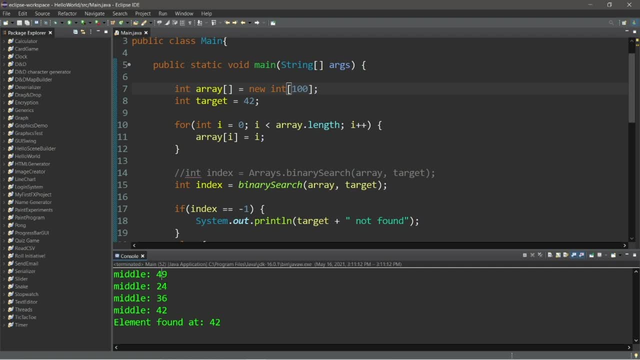 Okay, element found at 42. So it took us- let's see 1,, 2,, 3,, 4. Four steps- to find the number 42 within this array of 100 elements. Now let's increase the size, because binary searches do extremely well with large data sets.